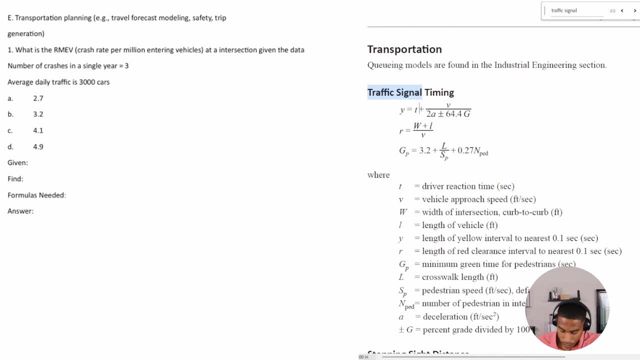 is given. Okay, so the number of crashes in a single year- just highlight this stuff in green. This is good information for us- And the average daily traffic. Those are the two things that are given. All right, What are we trying to find? We're trying to find the crash rate per million. 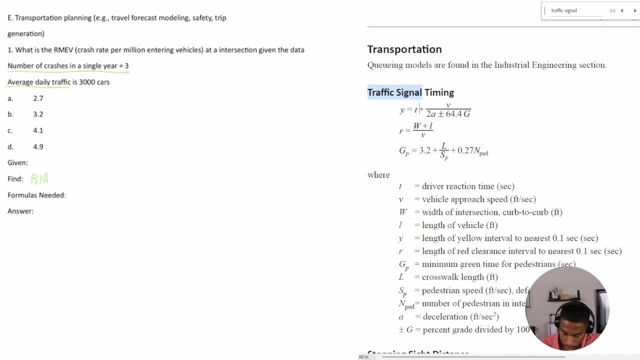 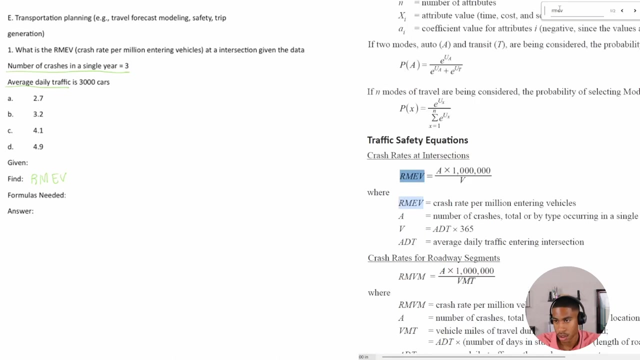 or the RMEV, And so are there any formulas needed for this? The answer to that is: I don't know what RMEV is, And I'm just going to do a search because I think that get me close: RMEV All. 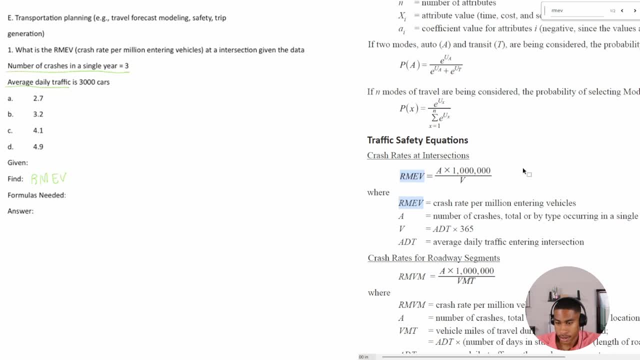 right. So now it's just a matter of looking at what they give us right. It's at an intersection. I think that's important to note, Because they give us a crash rate at intersections and they give us crash rates for roadway segments. So this is at an intersection. Okay, so the variables that. 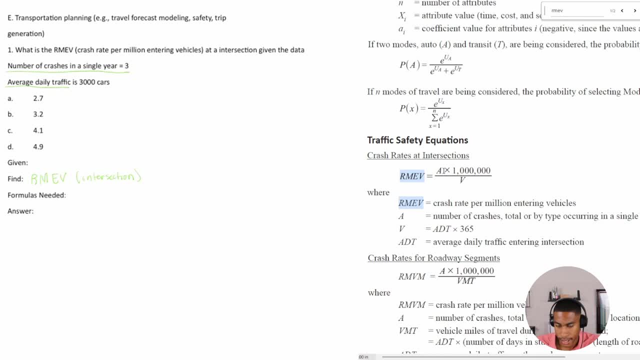 we need is A and V, So do we have A? A is the number of crashes in a single year at the location, So we have A, Which equals three. Okay, This information is given. This is why we write this stuff out. All right. 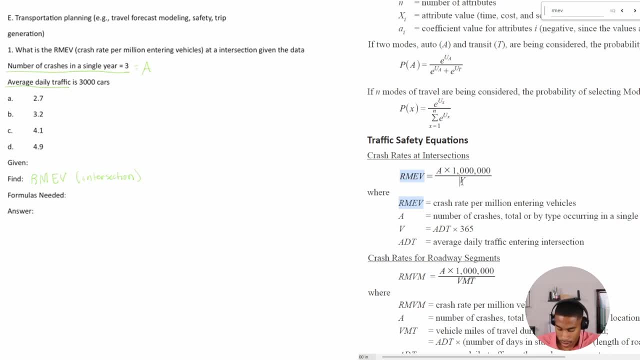 So what is V? V is equal to V is equal to ADT. Okay, times 365.. Do we have ADT? Because I don't know what V is, so I don't have V, But do we have ADT. 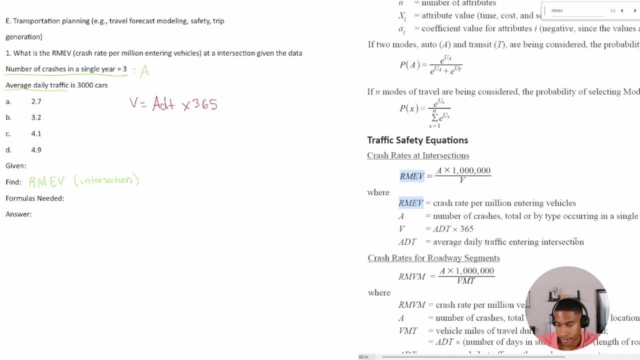 Well, ADT is the average daily traffic entering the intersection. Average daily traffic that we have is 3000 cars. So we do in fact have ADT. So now we can solve for V. All right, All right, So V is equal to. 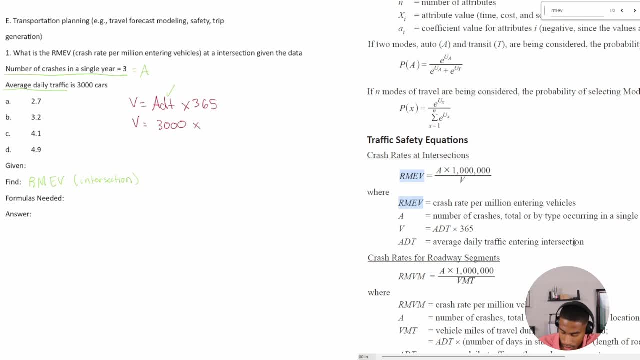 3,000 times 365, all right. so what is our V end up totaling to? so for V, we get one: zero, nine five zero, zero, zero, all right. so now we have B, we have a and we can solve for our crash. crash rate per million are our M e V, so our M. 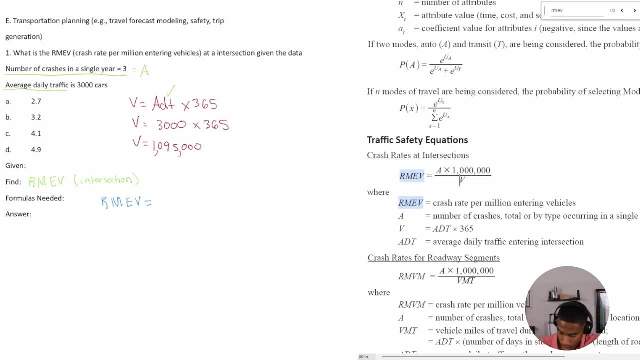 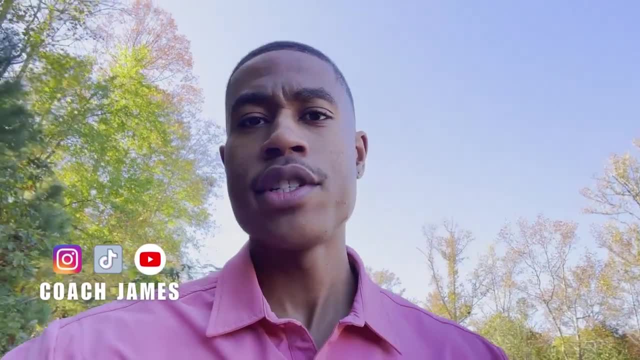 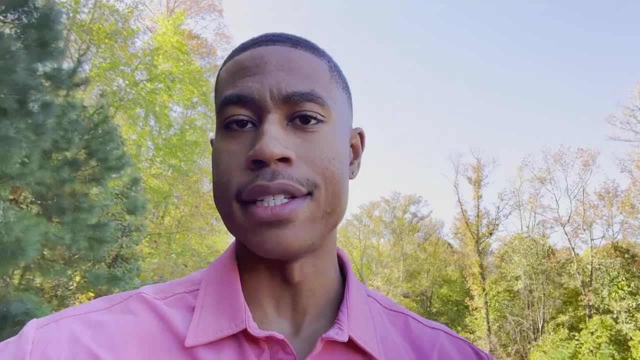 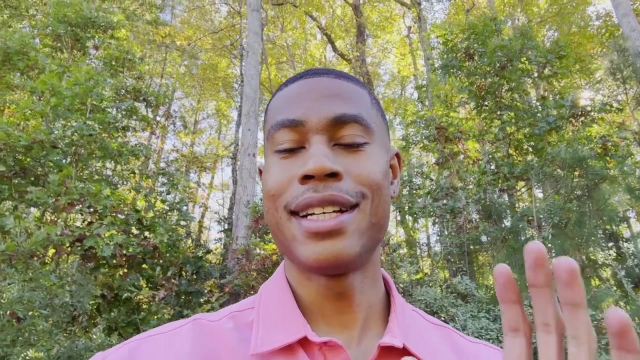 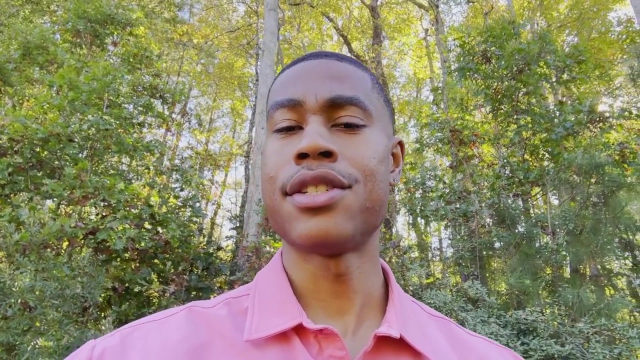